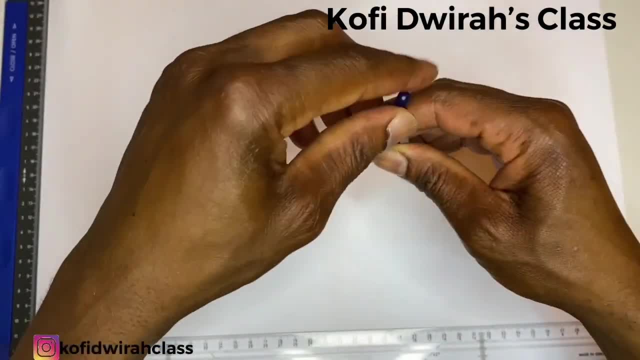 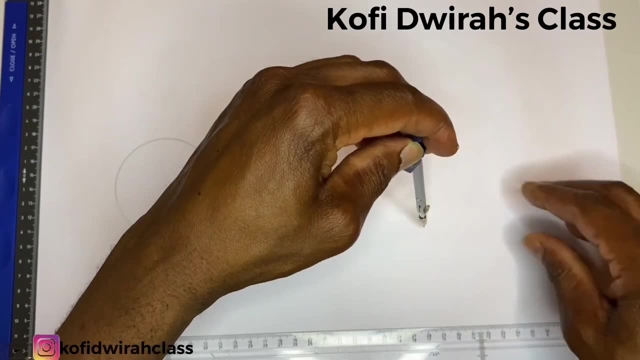 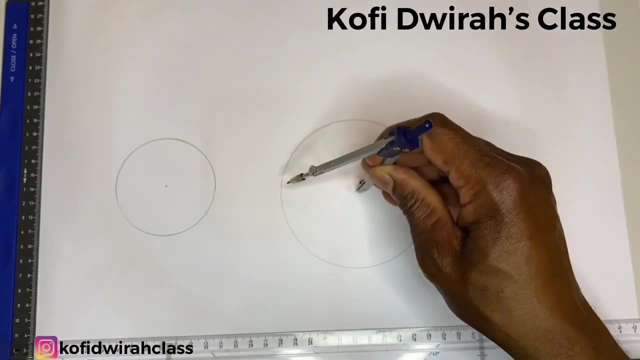 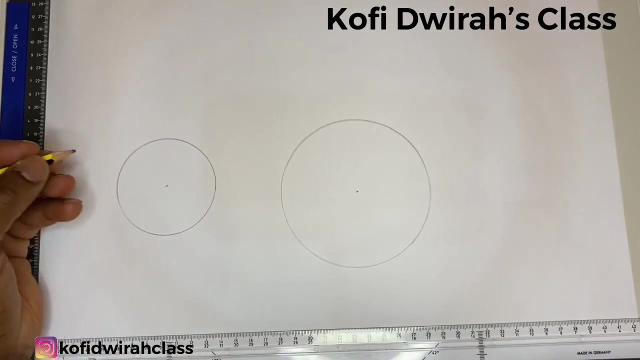 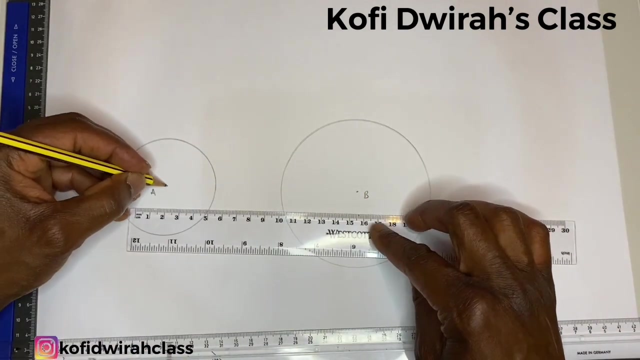 have the center. Then we draw our bigger circle, Draw our bigger circle, There is the center. So we have this point to be point A and we have this point to be point B. So you draw a straight line from A. So you draw a straight line from A. 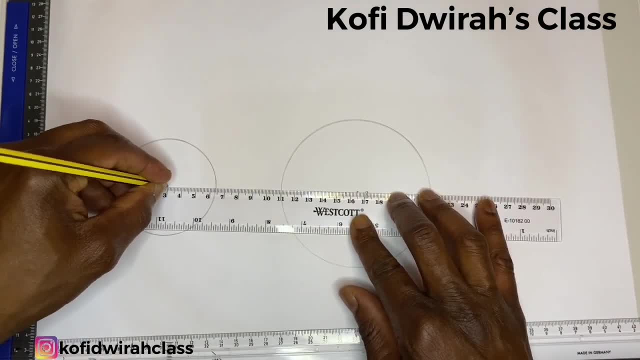 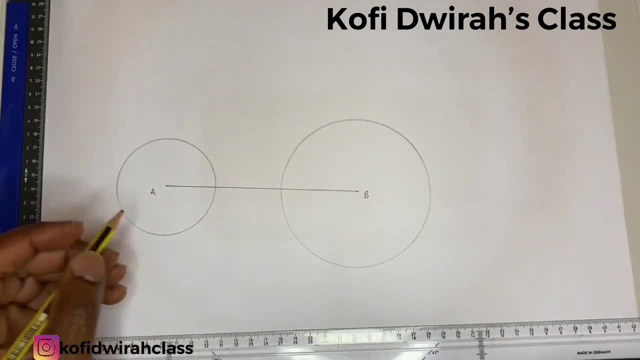 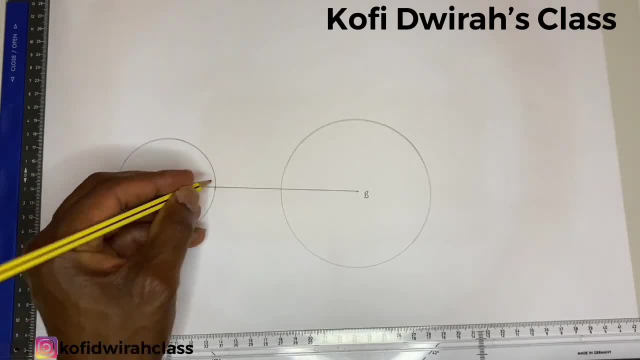 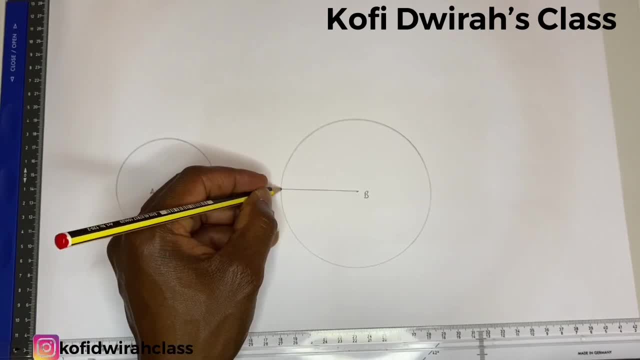 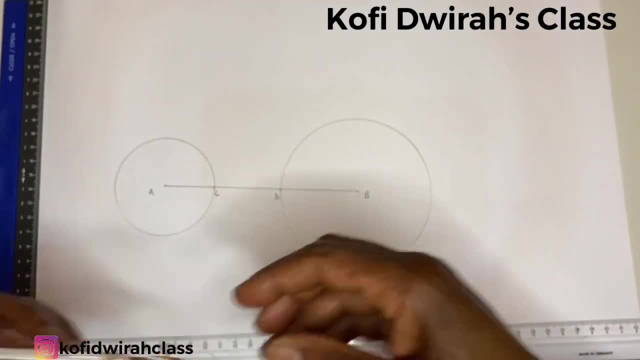 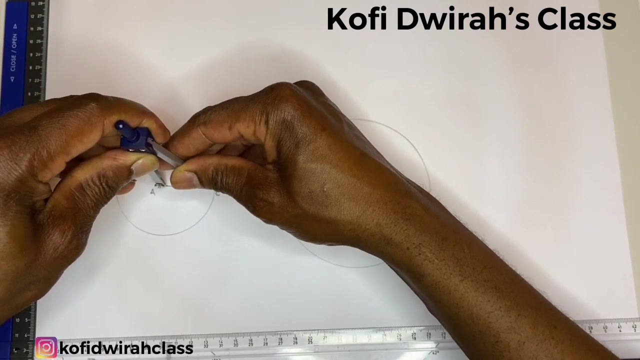 So you draw a straight line from A to B. So you draw a straight line from A to B And we have this point to be point D. Then you measure the radius of the smaller circle. The radius of the smaller circle, That is AC. 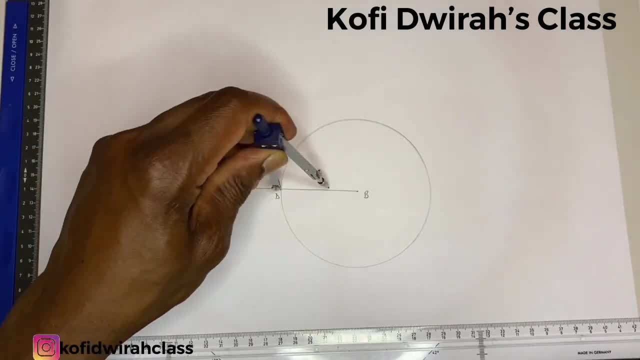 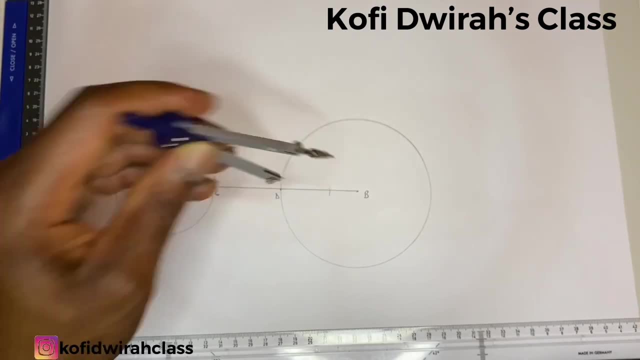 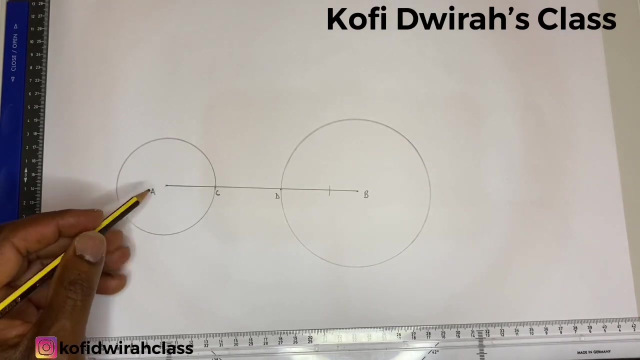 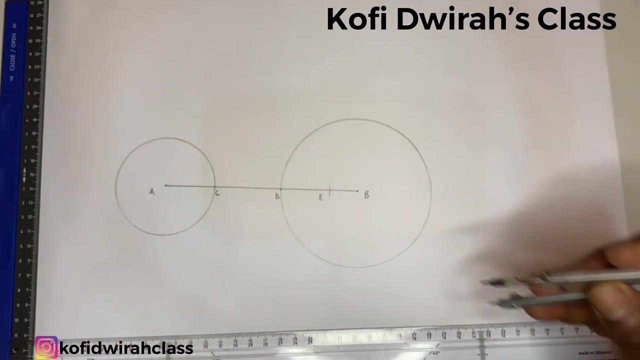 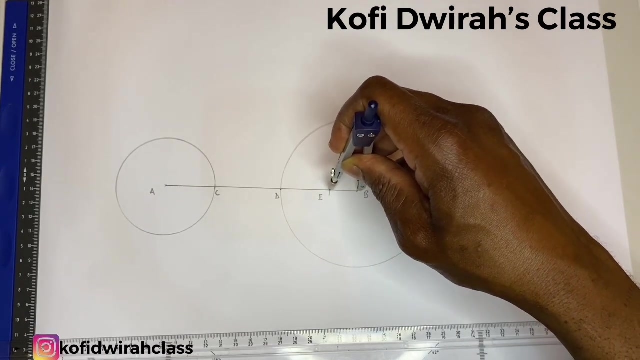 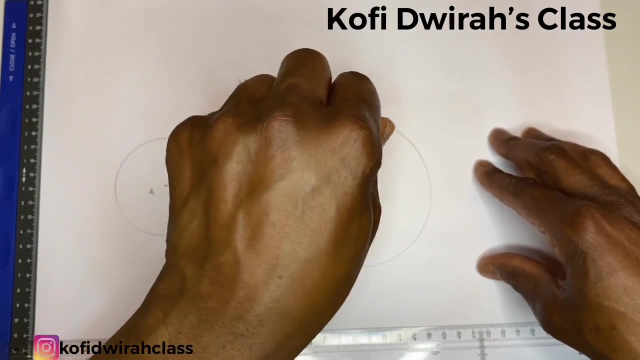 Then at point D you mark lie D, B, Then at point B, so we have point A, B, C, D, Then we have this point to be point E. So at point B you open the compass And you draw the compass to point E, Then you draw a smaller circle. 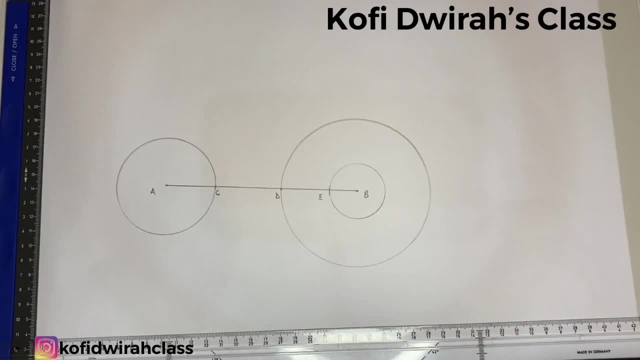 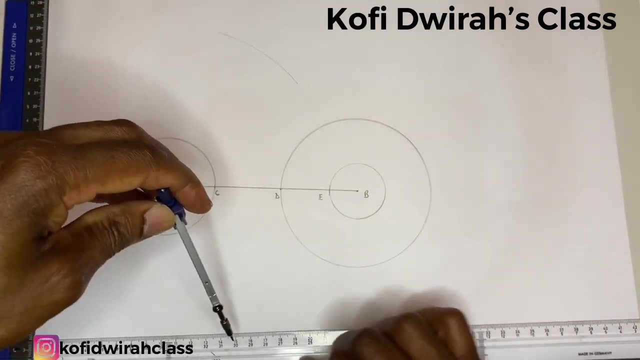 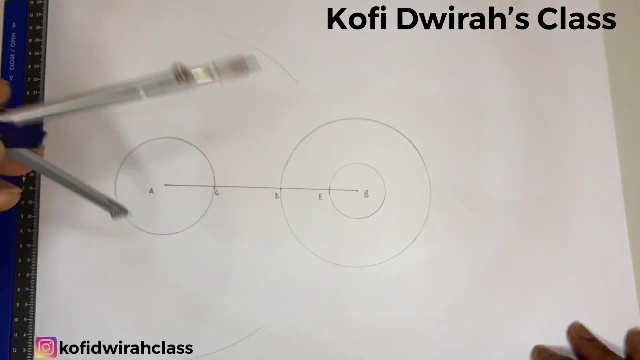 You draw a smaller circle, Then you bisect lie A- B, You bisect lie A- B. So at point A you draw your arc, Then at point B you draw your arc. You draw your arc like this. Then at point B you draw another arc. 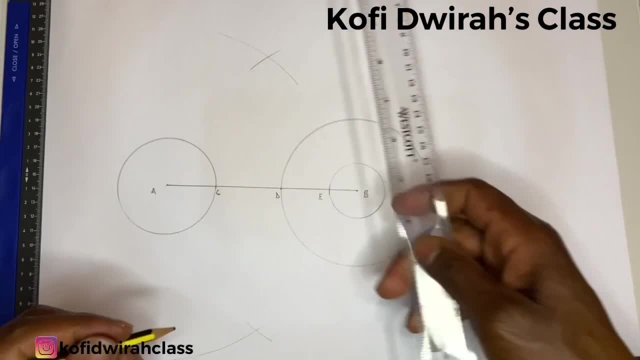 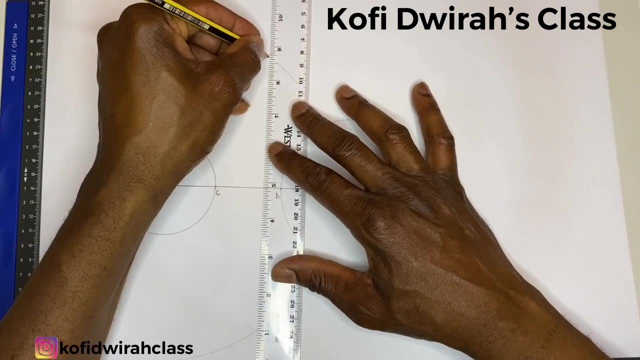 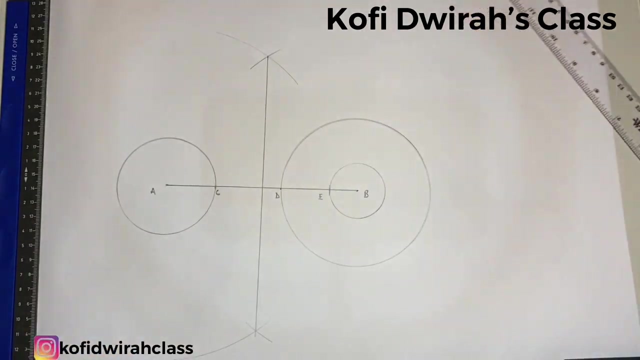 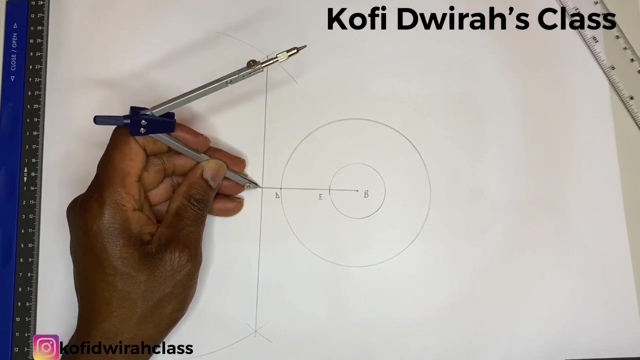 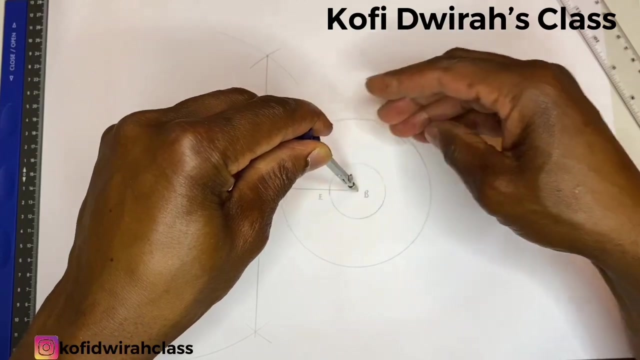 Then you draw your straight lie To get the center of lie A- B. Then you draw a straight lie. You draw a straight lie, Then that is the center. So with your compass And the center of lie A- B, You draw a semicircle that is from B. 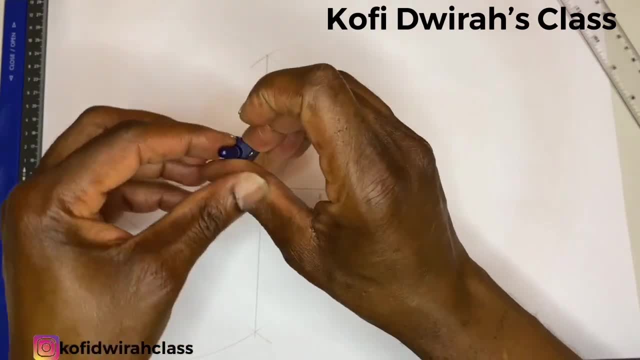 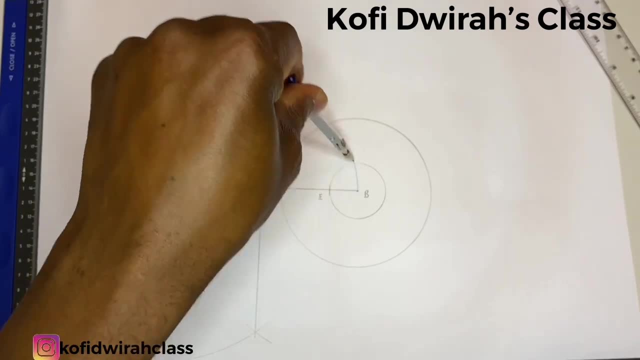 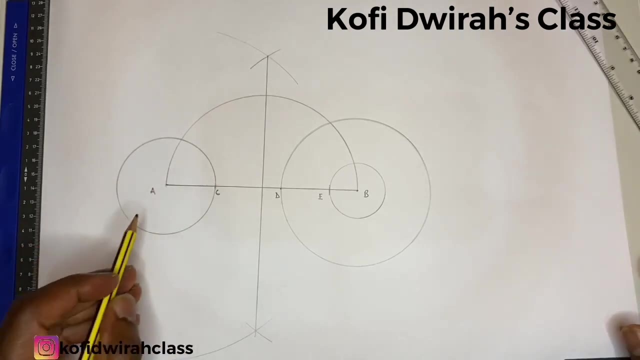 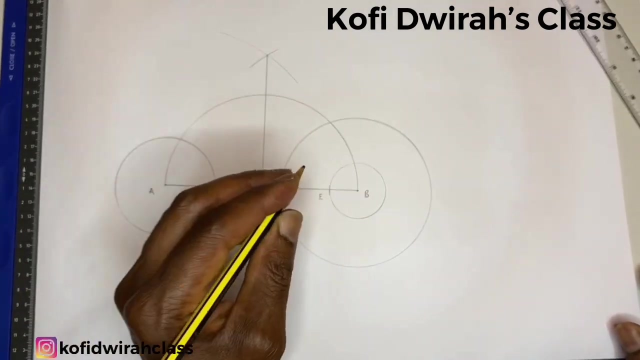 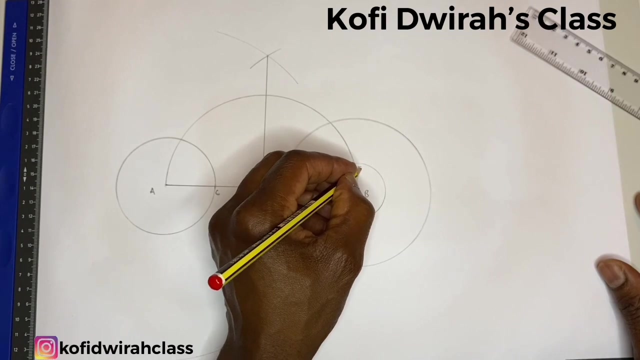 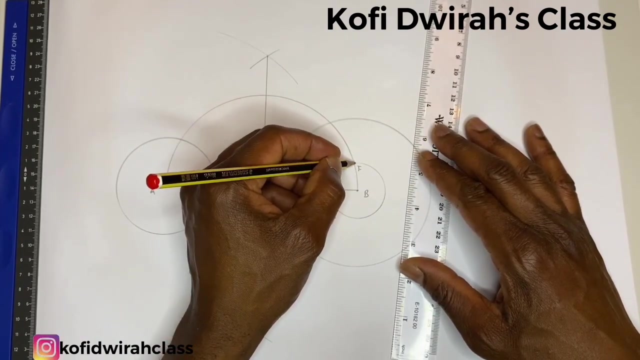 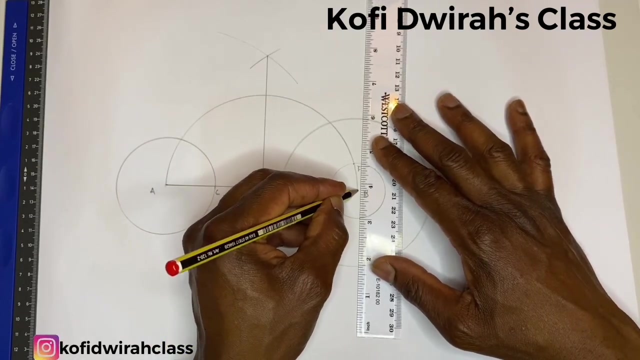 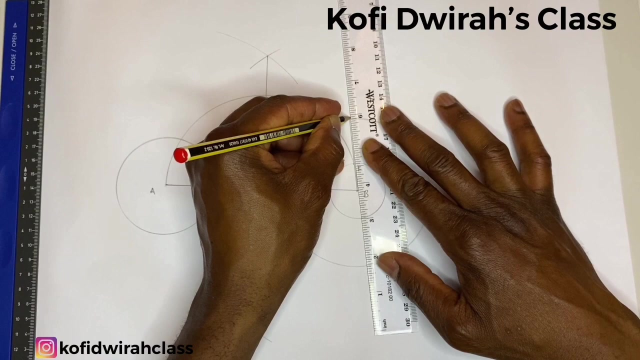 You draw a semicircle, you draw a straight lie. we have this point, we have point ABCDE, then we have this point to be point F here. so you draw a straight line from B through this point, point F, to the circumference of the bigger circle. so from here it goes like this: you draw a. 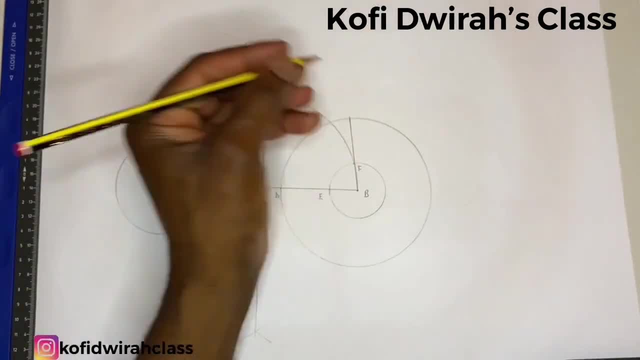 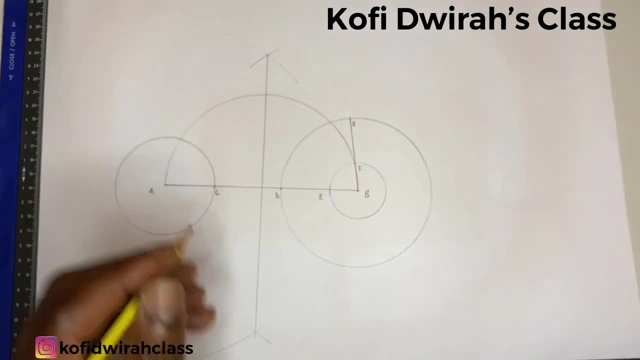 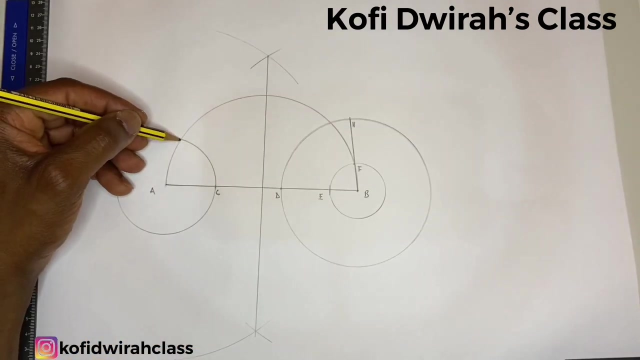 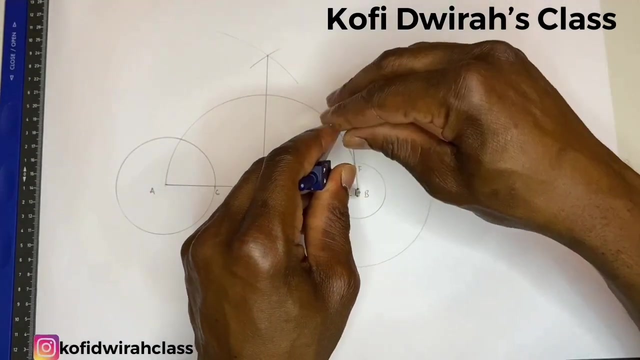 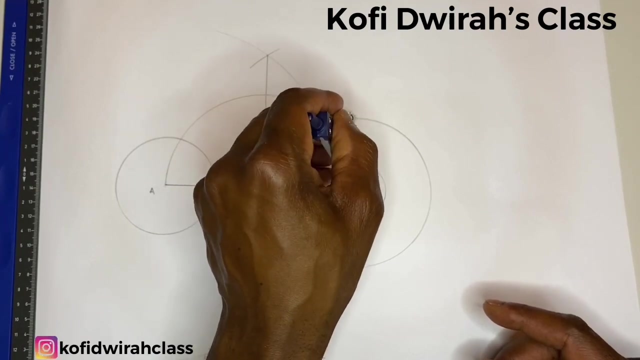 normal. so we have this point to be point. let's call it point H. so we have: this is a normal. so we need another normal here so that we can draw a common tangent to these two circles. so at point B you measure the radius that is from point AB to H. you measure this. then at point A you 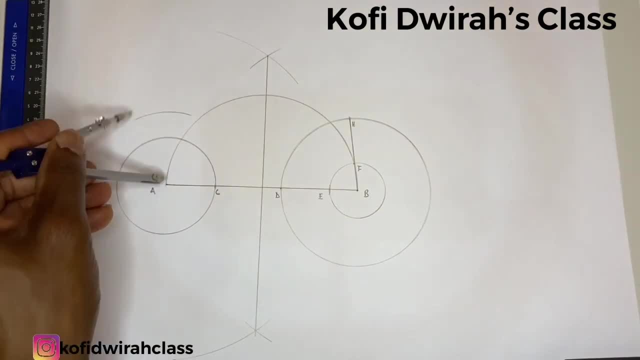 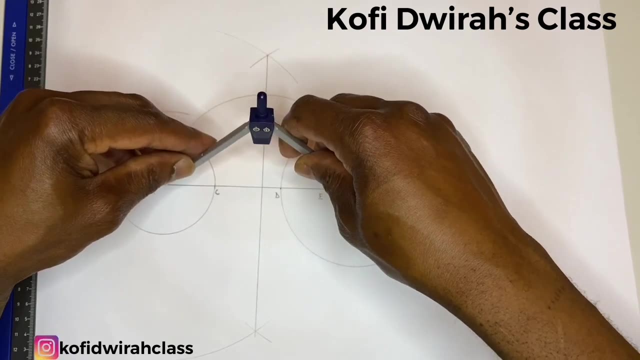 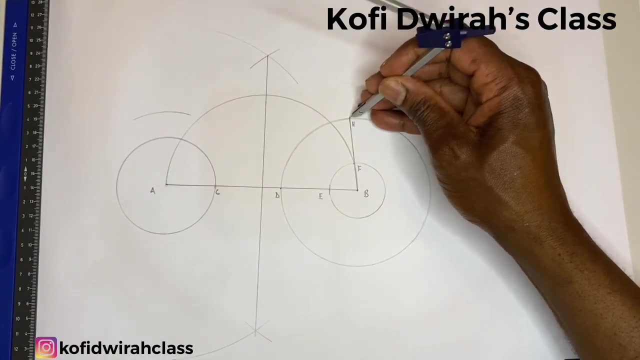 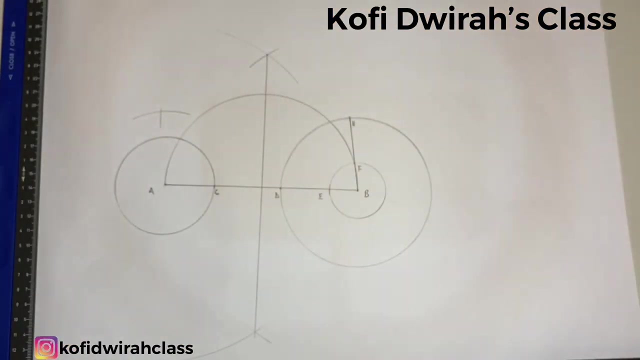 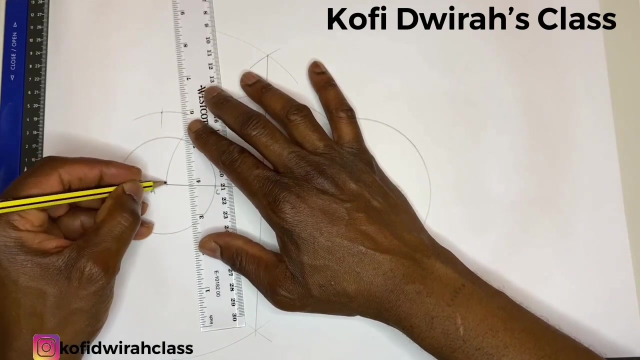 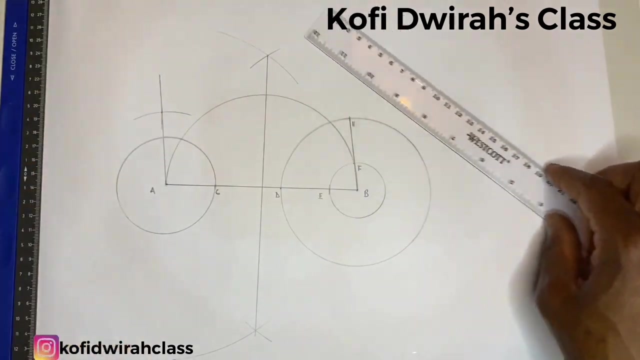 draw an arc. let's draw an arc. then you measure it like a be the radius of, like a, be good. then at point H you draw another arc. then so from here, then you draw a life, from a you can extend it to, to the base of B, to the ab position. so